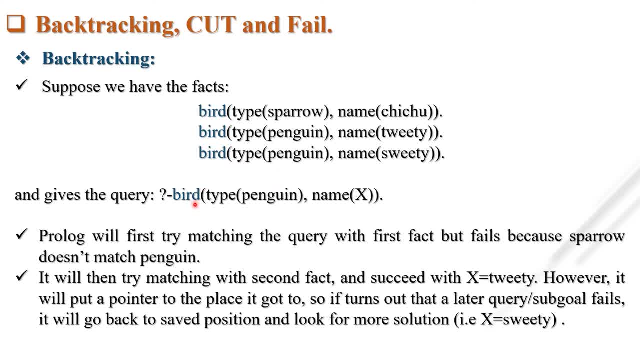 Suppose we give the query to the prologue, like bird type, Penguin, what is the name? OK, that's why I'm using here variable, So prologue first. Try matching the query with the first fact, but fails. Why fails Because this argument is not matched with Sparrow. 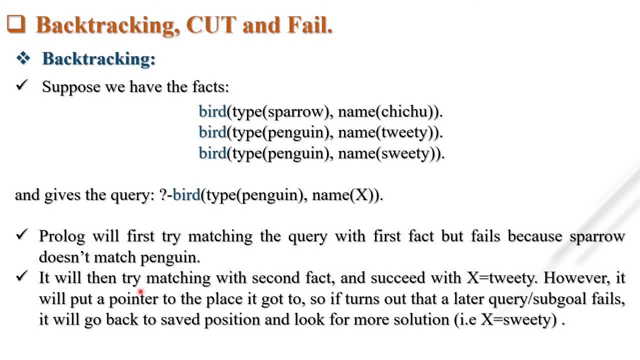 OK, so it will then try matching with second fact. OK, why second fact will be matched? Because the predicate we are using is bird. So first one is not succeed, It will try second one. If second one is not succeed, it will try third one. 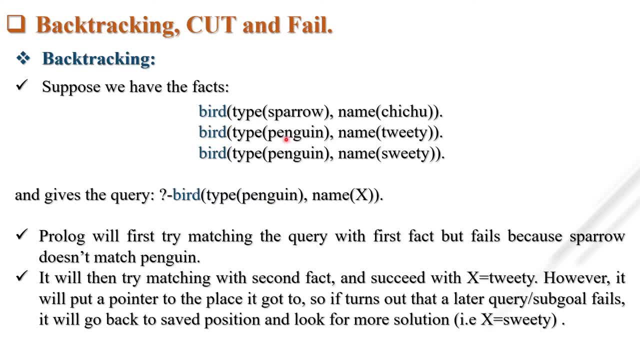 Now it checks this parameter is same: Yes, Penguin, Penguin. Then automatically the variable X contains Tweety. OK, so the value of variable X is Tweety. So whenever X equal to Tweety will stored in the variable X, it will put a pointer to that place. 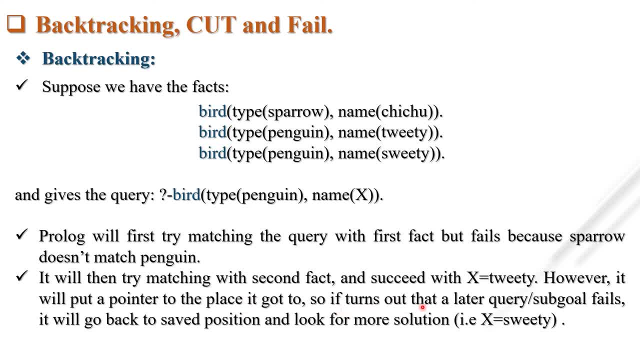 So if it turns out for later query or sub goals, If it is fail, it will go back to saved position and look for the more solution. That is X equal to Sweety. OK, suppose in this example, if I hit this particular query, it will give me the answer X equal to Tweety. 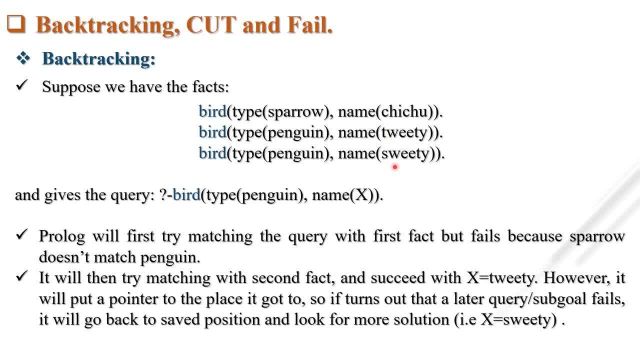 Then question mark. Why question mark? Because there is one more alternative will be there. So prologue keeps the pointer here. If I hit semicolon then it will give me the answer X, equal to Sweety. Why? Because I am not satisfying this answer only. 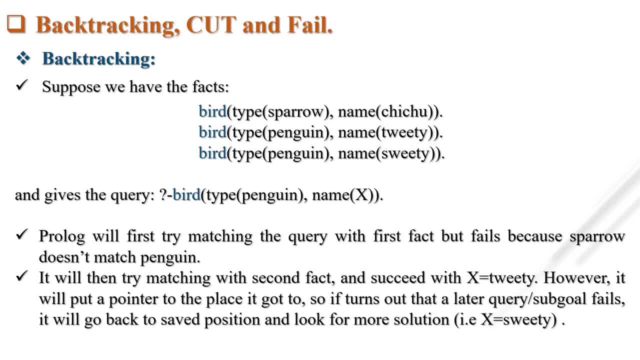 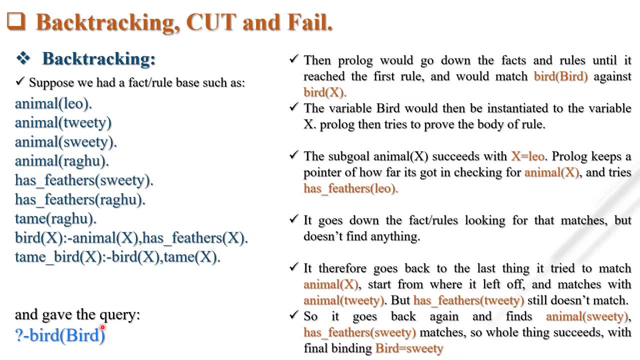 That's why I am hitting the semicolon sign. Semicolon means if there is another alternative of that particular variable, then it will source the answer. OK, Here it is one another example. suppose Leo is an animal, Tweety is an animal, Sweety is also an animal, Raghu is an animal. 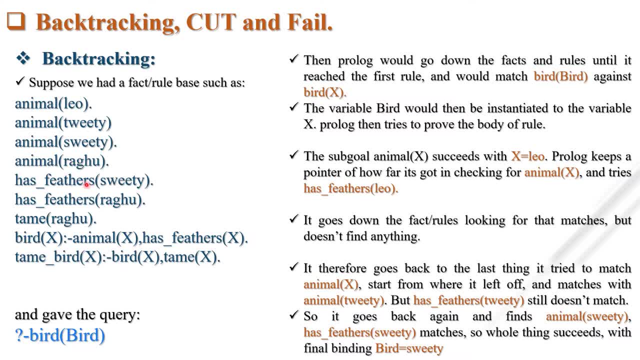 Sweety has feathers. Feathers means we can say that they have wings. OK, Raghu has feathers. Raghu is a tame And I have one rule whose head is bird and body is animal X comma has feathers X. And there is one another rule whose head is tame bird X and whose body is bird X and tame X. 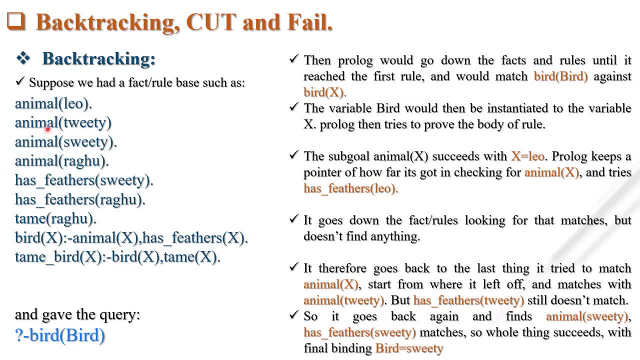 If I give the query after saving this program in the bin file with the extension of dot PL. If I hit this query, The answer will be bird bird, Bird bird. This bird is variable because first letter is starting with capital letter, So how will Prologue give the answer? 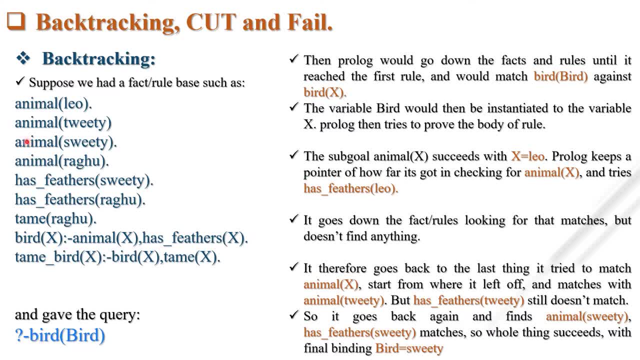 First it will go to check the predicate bird. Here it is bird. No, it always goes from top to down here. No, no, no, no, no, no, no. Here it is OK. So what is the value? or whatever the value of X is, it will be stored to this variable. 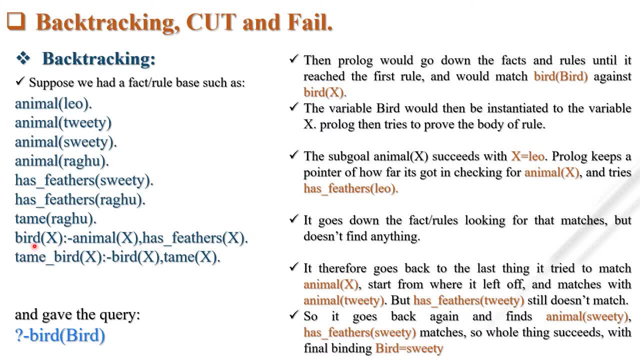 okay, now bird will be called. it have some rules? if it is true, then, and only then, the value of x will be given. so if i hit bird, variable bird, then it will go here first and then check animal x. so animal predicate first call where is animal from top to down here. so the value of x is. 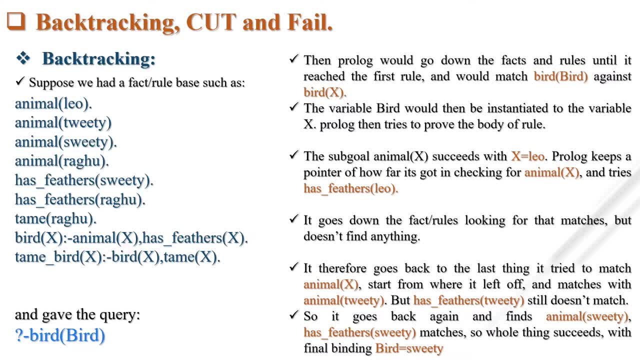 automatically. right now leo. okay, the value of x is right now leo, then it will check. this will succeed. then it will check. has feather leo, because the value of x is leo. okay, now we have to check. has feather predicate? it is there, yes, but the argument does not match, because it is a sweetie. 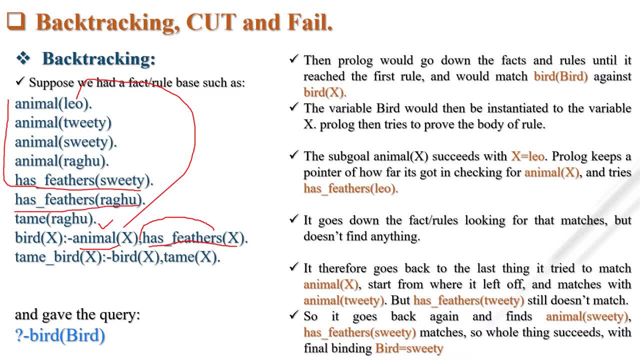 here also, argument is not matching okay, so so, so, so this is not successful. so prologue has inbuilt mechanism of backtracking. that's why it will go once again here and check for animal x, next alternative. what is the next alternative? first, in the place of x, we have leo. now it will be testing for tweety. now the value. 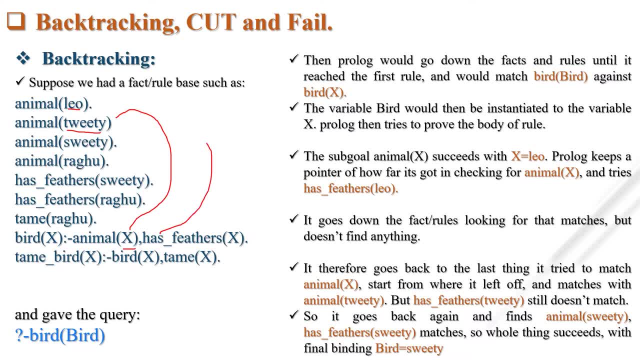 of x is tweety, now it will be checked for. has feathers tweety? no, no, this is also once again. this is not succeed and once again it will backtrack and try for the next alternative of the predicate animal. now the value of x is sweetie. okay, value of x is sweetie, now it will be checked for. next predicate that is: has. 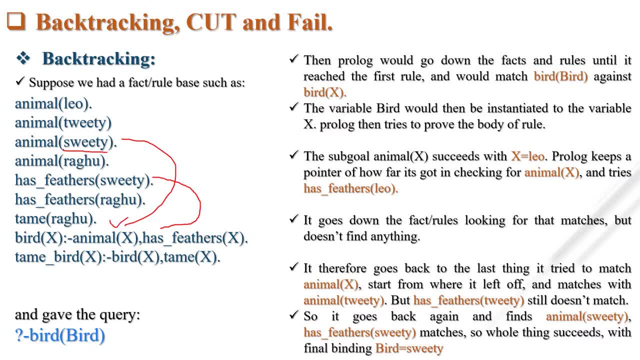 feather: uh, sweetie, yes, both are succeed. then the value of x is sweetie. you can say: the value of x and the value of bird is same. that's why here it has written that bird equal to sweetie. the whole explanation are already there in this right hand side. again you can go for it. let's see the next. 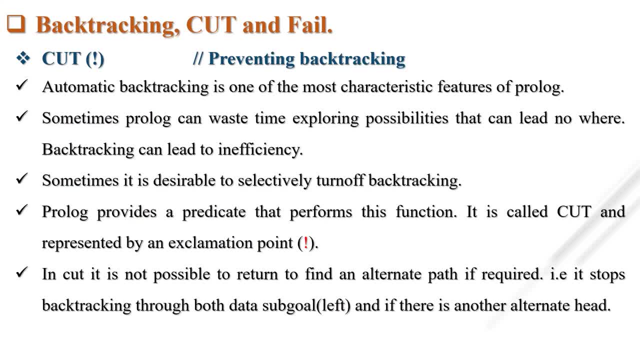 predicate that is cut. so this is most important predicate: cut, fail and repeat- which may ask in your gtu examination. also, it is important for your mid examination. okay, so what is cut predicate? it is used to prevent the backtracking because sometime prologue can waste the time by exploring possibilities that can lead nowhere. 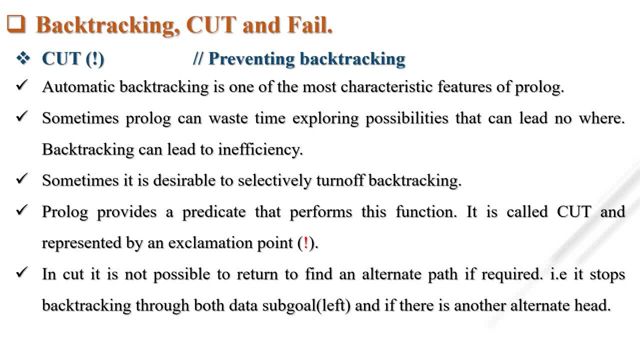 so backtracking can lead to inefficiency. so sometime it is desirable to selectivity, selectively turn off the backtracking. that's why this prologue provides a predicate that performs this function. this is called cut, represented by this exclamation sign. also in cut, it is not possible to return to find an alternate path, if required, that is. 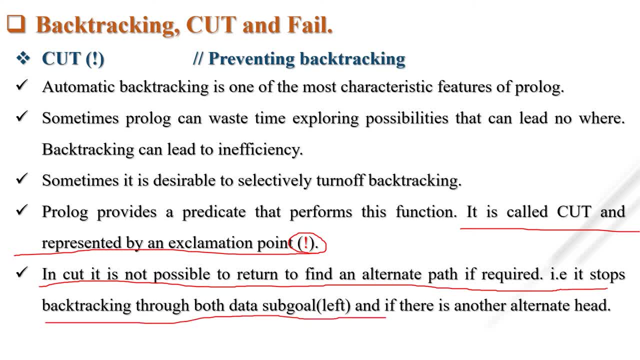 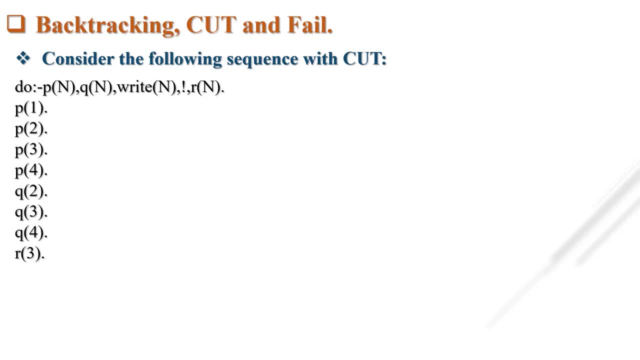 it stops backtracking through both data sub goal also, and if it is an another alternate head. let understand cut predicate with the help of example. consider the sequence where the value of p- suppose the value of p- is one, two, three, four. similarly, q starts with two, three and four and i start with three. 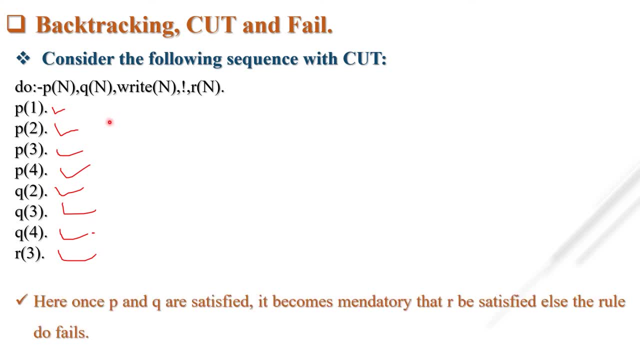 okay, so whenever i hit, whenever i hit, do so it will first go to p of n. what is the value of n first? p predicate will be checked. so the value of n is this one: n will be stored. uh, sorry, one will be stored in the variable n. okay, so p will succeed. 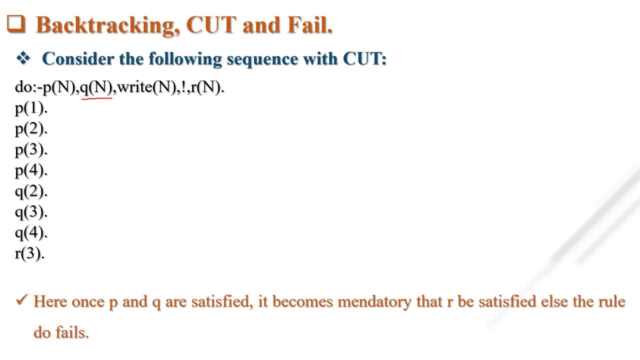 then there is a comma. there is a next statement, that is q of n. what is the value of n one? is there is any q of one? no, q of two and q of four is all there. okay, so this will not succeed. so, as we know, we have to backtrack. 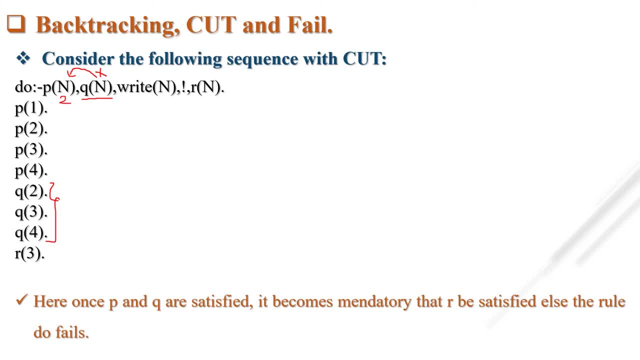 now the value of n is two, because u of two will be there. this value is stored in variable n. okay, now the variable- sorry, variable n value is two. now it will be checked for q of n if there is any predicate for q of two. yes, this also succeed, this also succeed. so what is the output? 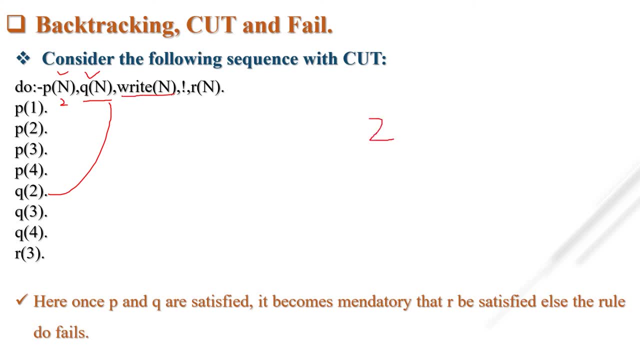 right n. so the output will be: first two. okay, so these three statement are succeeded. now cut predicate: succeed what this cut predicate do now. you are not able to backtrack any of these three statement. also, you are not able to backtrack these two. okay, whenever we print this two. 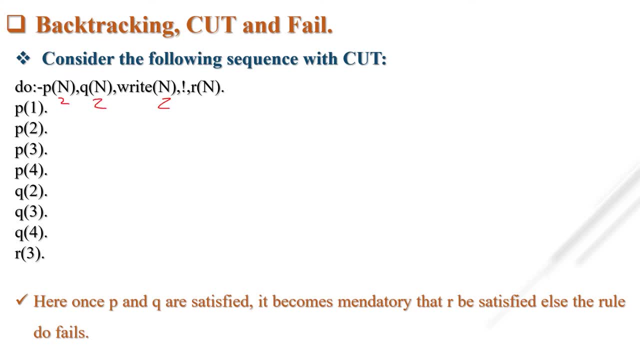 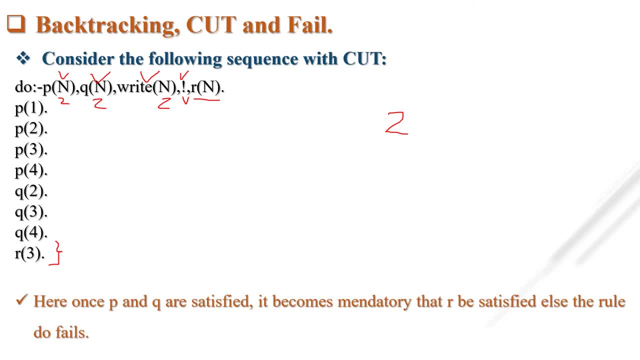 this will succeed. now we are not able to backtrack because cut predicate will called earlier. okay, before r, there is execution of cut predicate. that's why we are not able to backtrack and change the value of n to three. okay here. once p and q are satisfied, it becomes mandatory that r be satisfied. 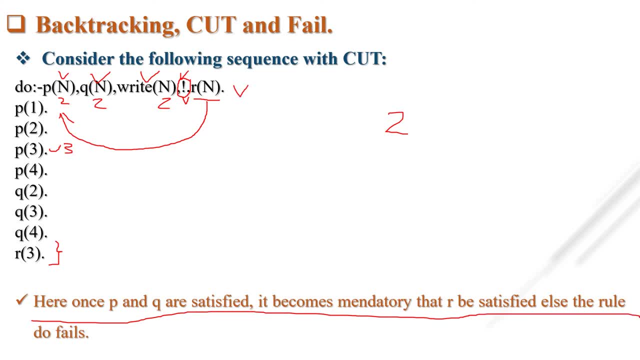 else the rule do fails. so this rule is not successfully satisfied. okay, so whenever i hit the do button- sorry, not do button- if i hit do atom, then what is the answer? it will be printed to and then it will be: say: no, why? no, because this is not succeeded. 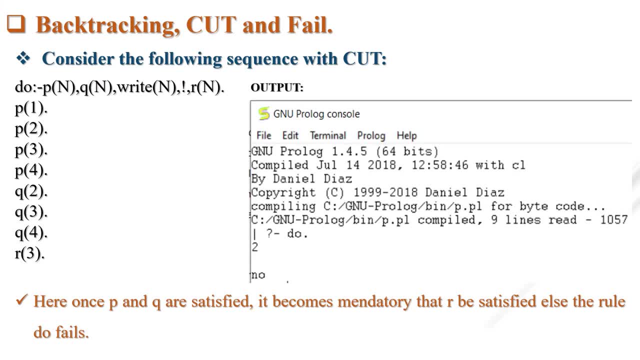 let's see the output. okay, this is the output. when i hit do what is the answer? only two, because we are not able to backtrack from here. why we are not able to backtrack? because that will be executed before this field call. let's understand with another example, without cut: okay, 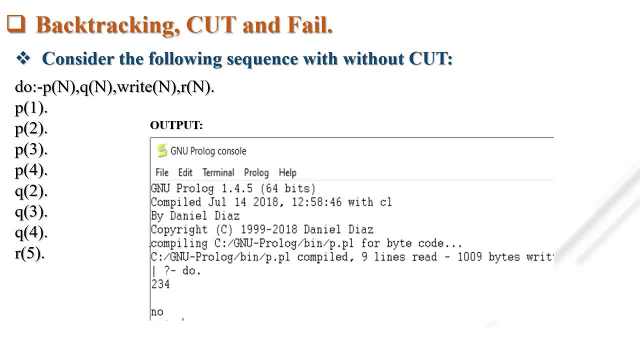 so here there is no cut in the in this prolog program. what is the value of p of variable n 1? this will succeed it then. is there q of 1 in our program? no, it is not succeeded. that's why it will backtrack and change the value of 1 by 2, because it is not succeeded. 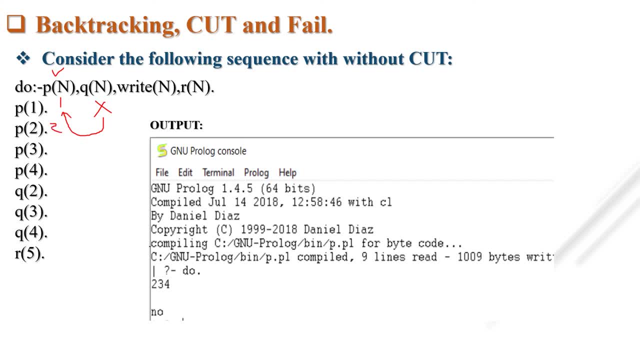 so we are not able to backtrack because p of 2 will be there. so the latest value of n is 2. q of 2 will be there. yes, it is. then what is the output? we have to print? 2, so 2 will be the output. 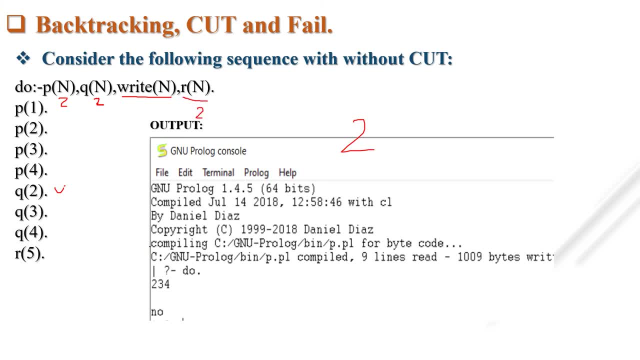 okay, then r of n is succeeded or not. it will be checked. is there is any r of 2? no, now backtracking will happen because there is no cut before the r of n, so prolog backtracks wherever it succeeded. previous predicate: that is 2, now the value of n. 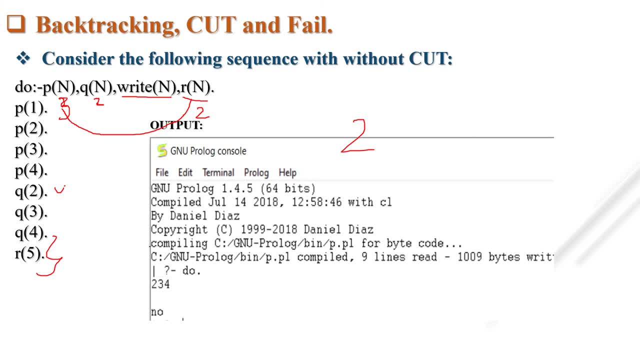 will be 3.. is there q of 3? is there in our program? yes, so the value of n is 3. it is also succeeded. this is also succeeded. now what is the output? 3, 2 and 3 is the output. Now it will be checked for R of n. 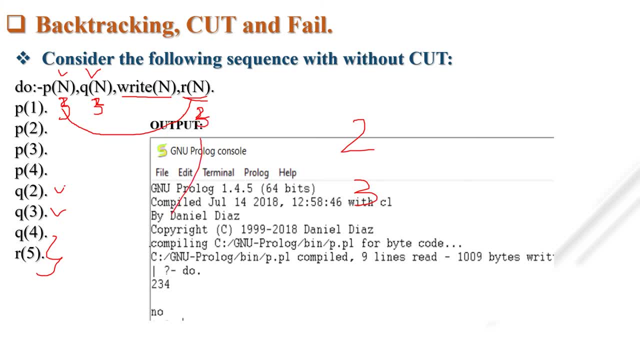 What is the value of n 3.. Is there is R of 3 in our program? No, Once again it will backtrack. Once again it will backtrack and the value of n will be changed to 3.. Because P of 3 is there. 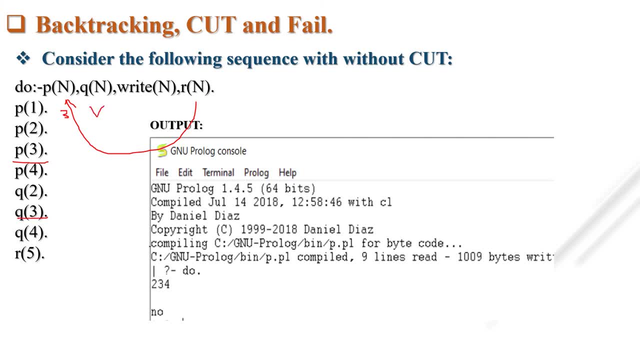 P of 3 is there. Yes, this is also succeeded, Because the value of n is 3, we are also 3.. That's why it is succeeded. Then we have to write the output 3.. So what is the output? 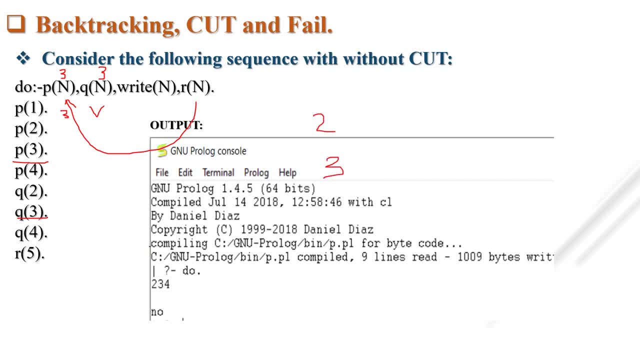 2, then 3.. Okay, But R of 3 is not there. Similarly, R of 4 is not there. P of 4 is there, Q of 4 is there. So 4 will be the answer. Suppose now this will print it: 2,, 3 and 4.. 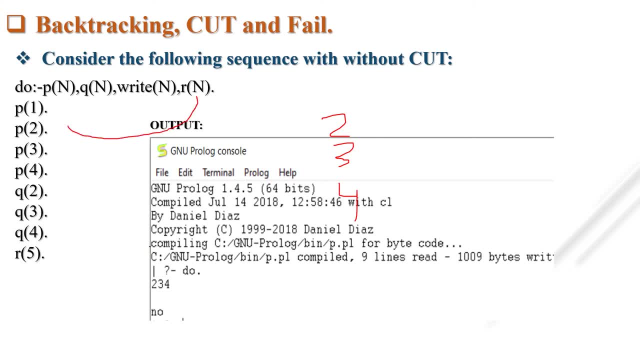 Okay, Now once again, it will backtrack, Then check that. is there Any other alternative? for P? No 4 is the last one. That's why the answer is no. But what is the output? 2, 3 and 4.. 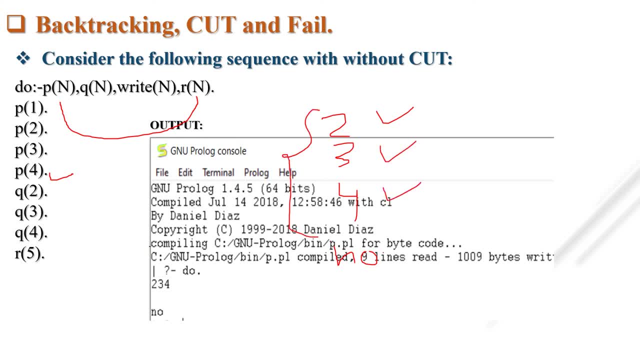 Why we get this output? Because we are able to backtrack in this program. If I put cut here, then I am not able to backtrack. That's why in previous slide, what is the answer? Only 2.. So this is the difference between. 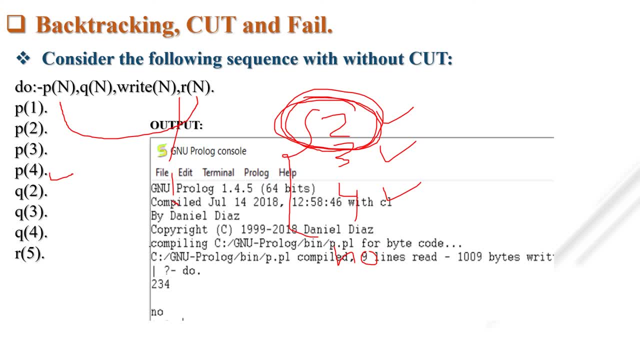 when we put 2, when we put the cut before the predicate. and what is the answer when we will not put the cut before the predicate? Okay, So the answer is 2,, 3 and 4.. If you put the cut before this, R of n. 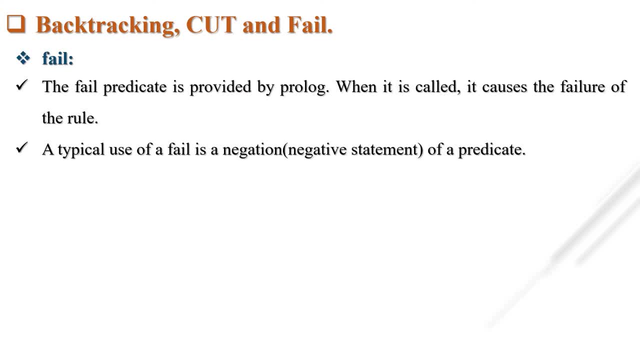 then what is the answer? Only 2.. So next predicate is fail. The fail predicate is provided by prologue. When it is called, it causes the failure of the rule, So it will always give the negative statement, even if it is true. 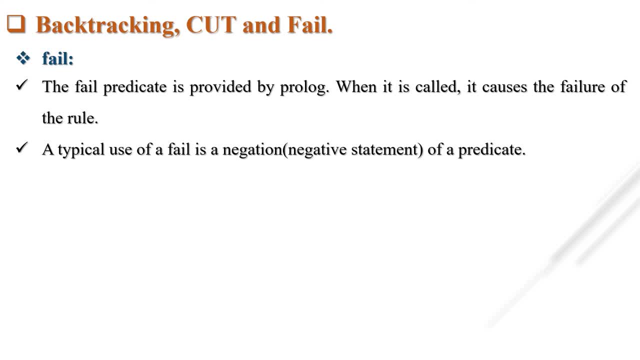 Okay, So typical use of fail is a negation, that is, negative statement of the predicate. Let's see the example. This is a prologue code with the fail predicate We are using here: fail predicate: Here it is. So whenever I hit z. 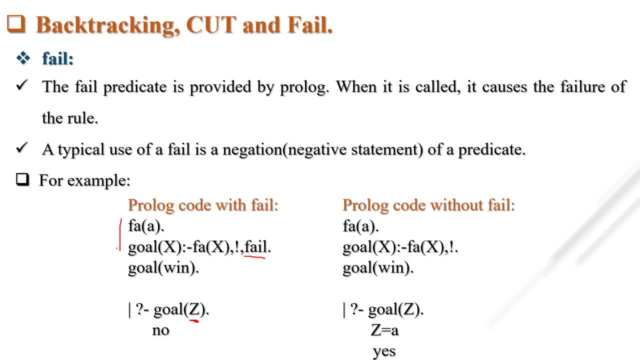 goal z. first it will say it will go here and whatever the value of x is, it will be stored in z. Okay, Then in the body of goal, fa will be called this one. So what is the value of x? 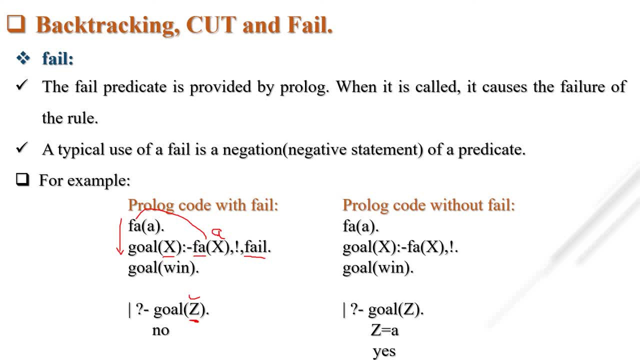 a, Now cut will be executed. Cut means what We are not able to backtrack anymore. Okay, And then fail will be executed, Even there is a value that is z equal to a. what fail gives the answer No, Why? 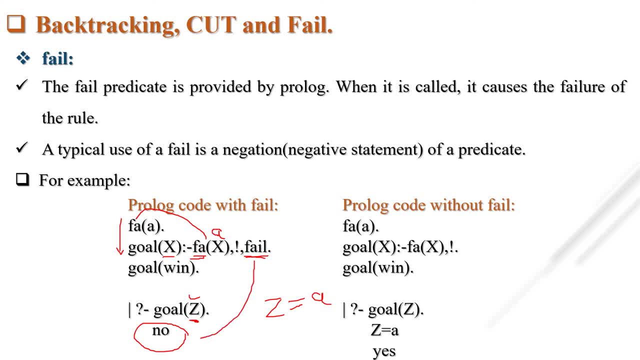 Because fail predicate is executed. Suppose we are taking this similar example without fail, then what is the answer? Answer is a, Because we see here that the value of x is a. Then also, if this fail predicate is executed, then it will always give the negative statement. that is no. 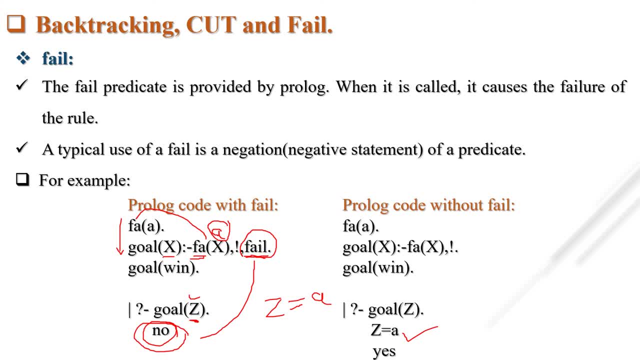 Even there is a value of z Here. if we delete the fail predicate, then it will give the answer, that is, z equal to a and yes. So fail predicate gives always negative statement, even if it is true or if even the body of the rule is succeeded. 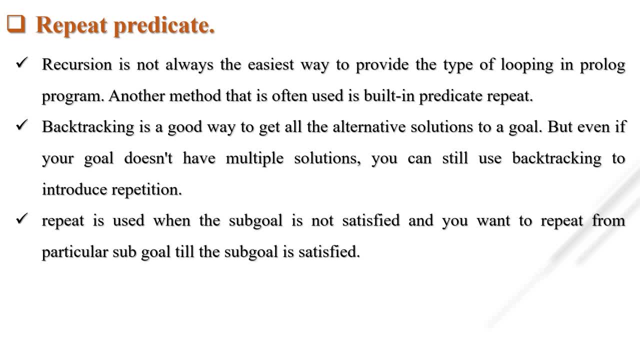 Okay, The last predicate is repeat predicate, So recursion is not always the easiest way to provide that type of looping In the prologue program. there is one another method that is often used to build in predicate that is repeat. So backtracking is good way to get all alternative solutions. 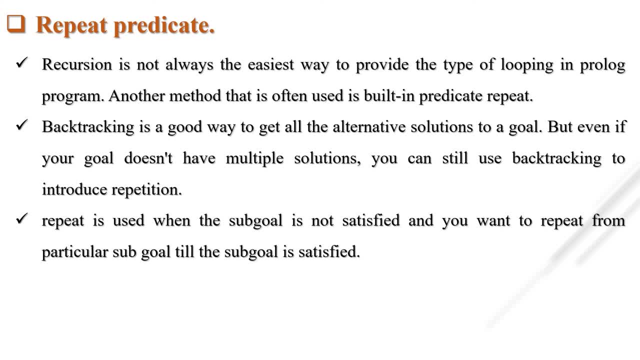 to a goal. But even if your goal does not have multiple solution, you can still use backtracking to introduce the repetition. So repeat is used when the subgoal is not satisfied And you want to repeat the particular subgoal till the subgoal is satisfied. 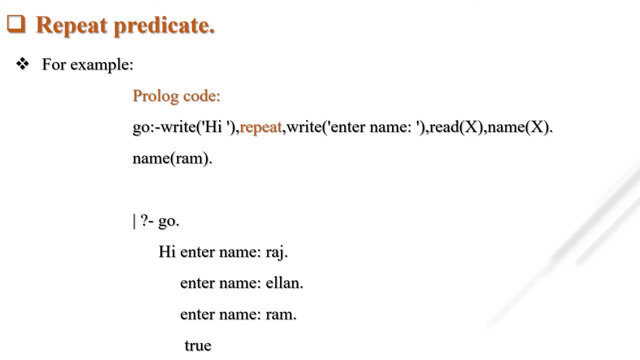 Let us see the example of repeat predicate. Okay, We have one program of repeat predicate. Here it is a program and here it is an output. First, what we do: we hit the go atom with the dot. Then this will be executed high. 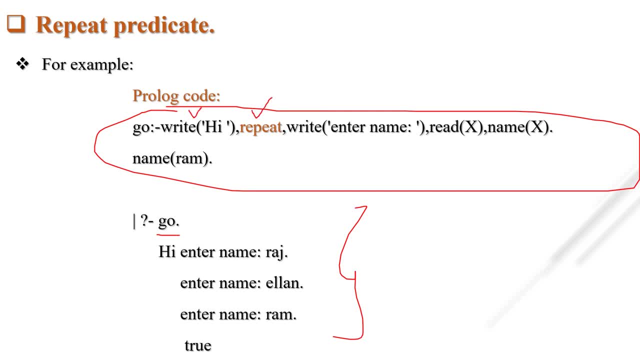 Then repeat predicate will be executed. Then the prologue will ask the question that enter the name Here. it is Suppose I am entering Raj, So this will succeed. This statement is also succeeded. The value of x is Raj. Now the name predicate will be called with the argument Raj. 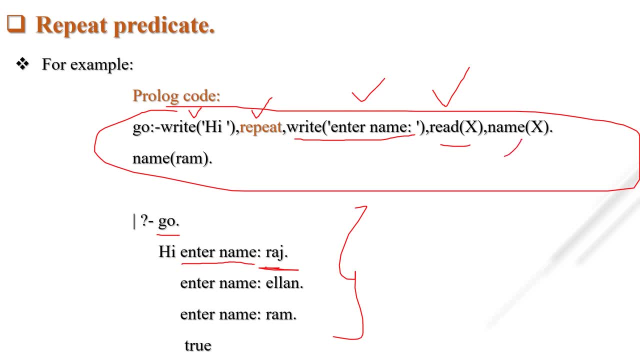 Is there any fact in our program with name Raj? No, Here it is name Ram. So this is not succeeded. So what repeat predicate will do If any subgoal is not succeeded? any subgoal is not succeeded, whole program will repeat it from here. 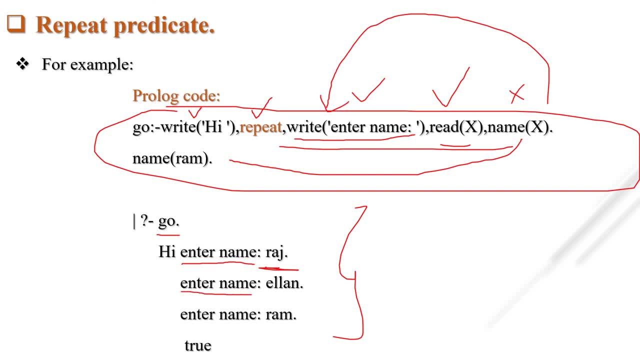 You can see. once again they are asking the name. I am writing Alan. Alan will be stored in the variable x. Now it will be checked with the name Alan. There is no fact, So once again it will go from here. Once again they will ask to enter the name.